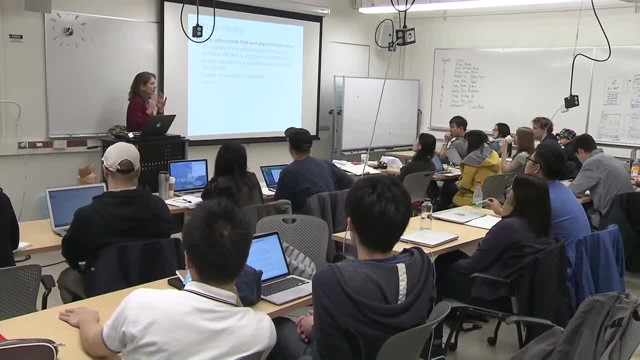 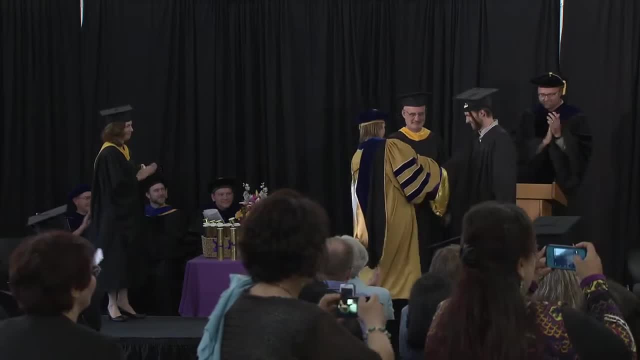 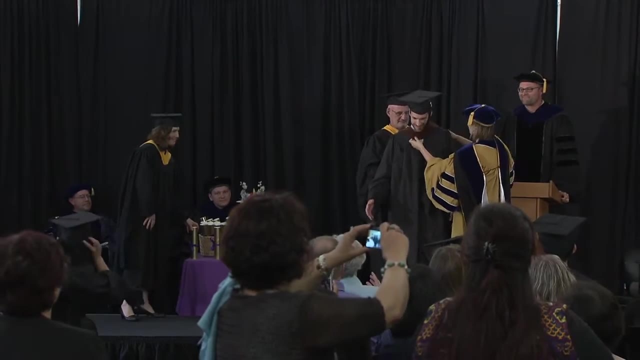 aspects of traditional visual or interaction design in their curriculum, and that's something that we do focus on. In August 2014,, the University of Washington's exciting new master's program, MHCI plus D, recruited its first group of graduates. The biggest word I hear from them is confidence, Confidence. they feel in the interview like 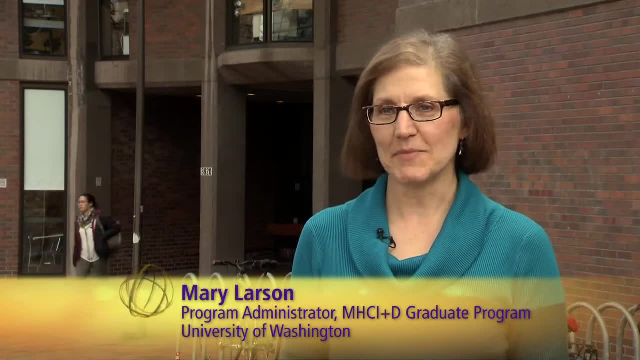 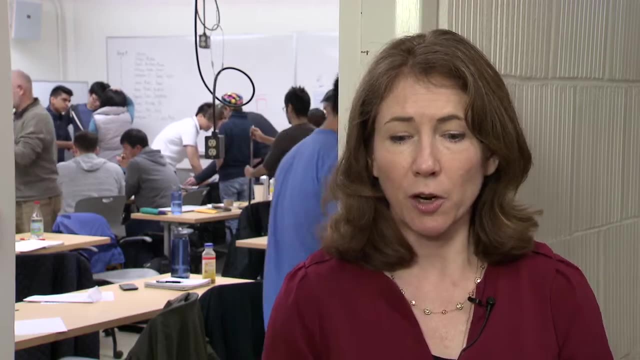 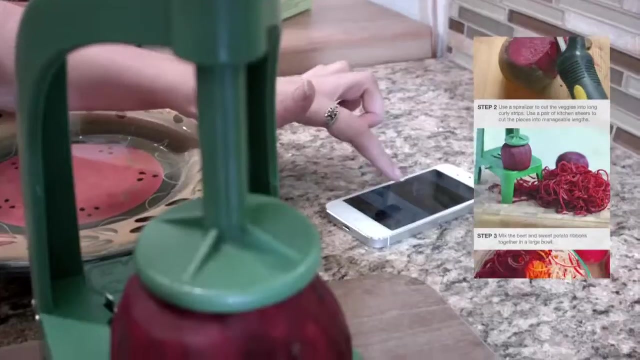 they really understand the interview questions or the subtleties behind those questions. We've got people who are working at Amazon, at Microsoft, at Facebook and a range from, you know, full-time roles to freelance roles to contract roles. This unique program is a product of several disciples merging together in response to 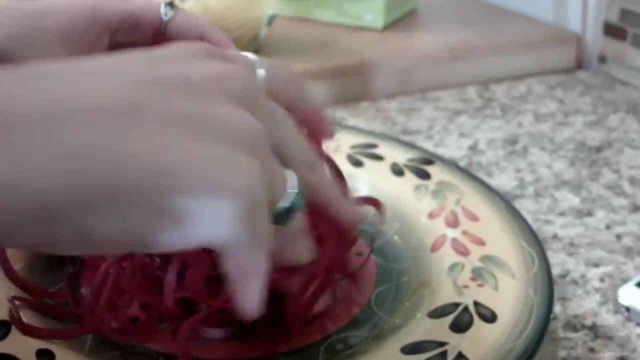 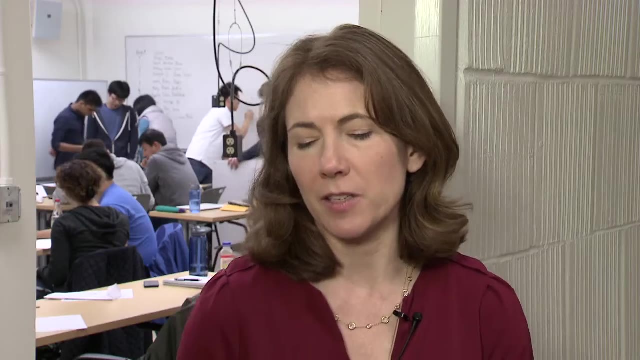 the demand for cutting edge technology and creative education Aesthetically pleasing interface. Part of the original proposal was to recognize that there was a growing demand for this kind of a degree, not only from students, but also from industry looking for people to hire. 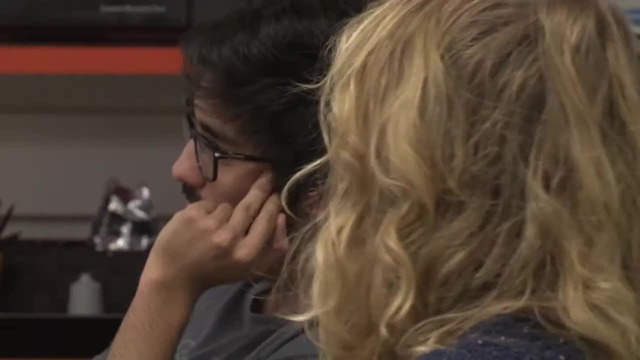 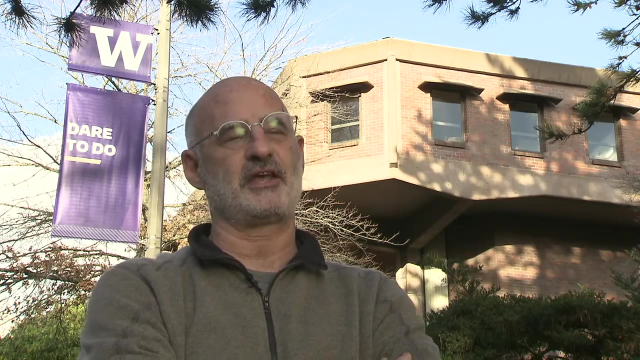 This is an immersive, really intense 11-month start-to-finish kind of experience, and that's a different style than many other graduate programs, Very exciting and, as I said, engaging. These students have signed up for a specialized education that will prepare them to succeed. 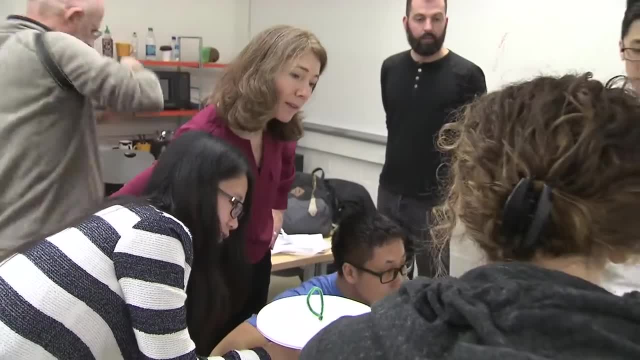 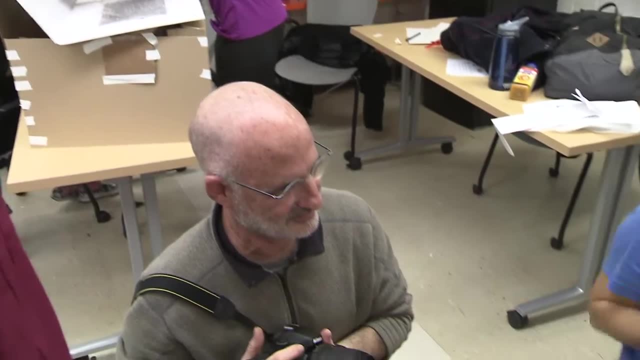 in the competitive tech industry. Generally, what we do is a mixture of critique of projects and work that they've done in previous classes and then an in-class kind of hands-on exercise on some new topic. So I'll begin by defining our problem stage. 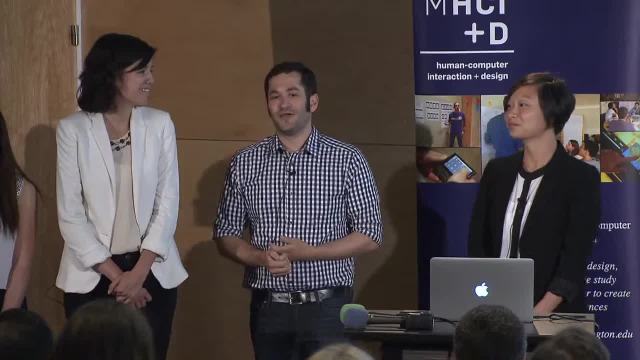 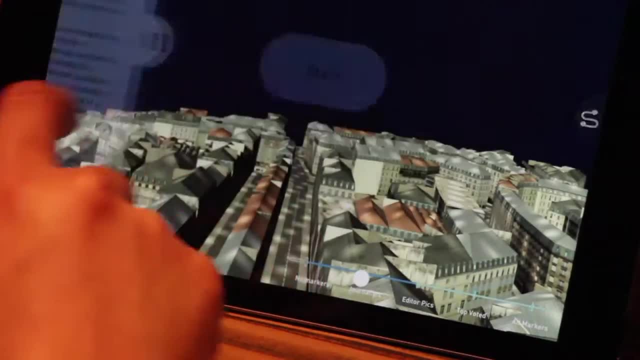 MHCI plus D has drawn a diverse crowd, with prospective students coming from a wide variety of backgrounds and demographics. There's a whole group of design background, including architecture, graphic design, even fashion design, And then there's also the technological people, The computer science. 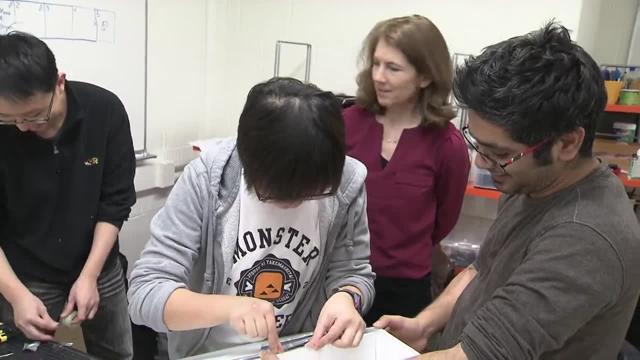 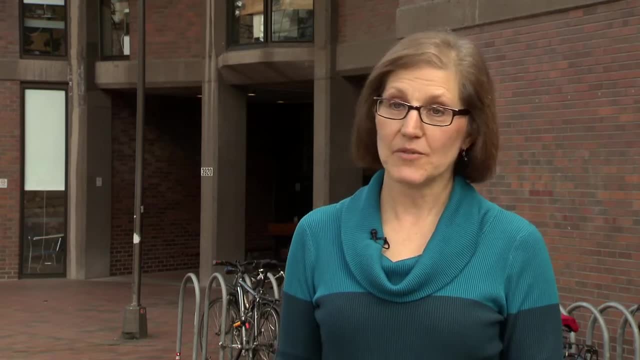 Computer science people. And then there's people- I just have to call them people people. We have age range, I think, from 23 to 53.. People right out of undergrad, and then also people who are mid-career or have had a few. 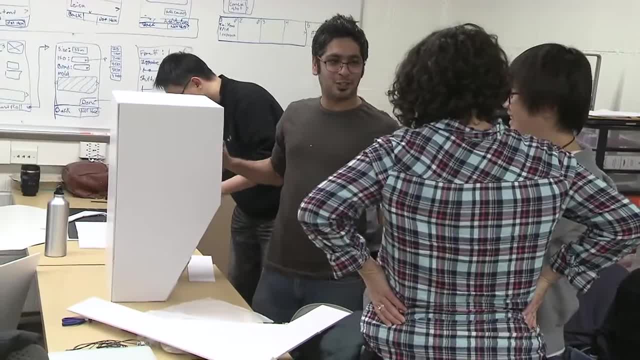 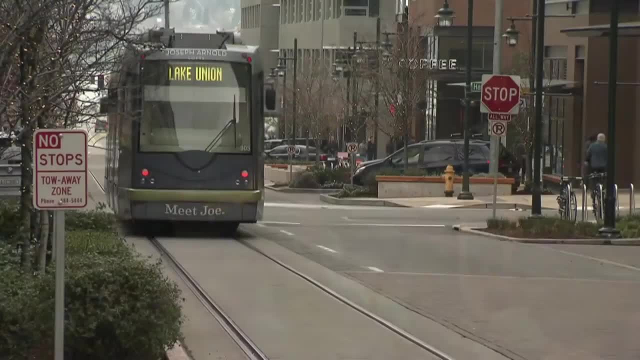 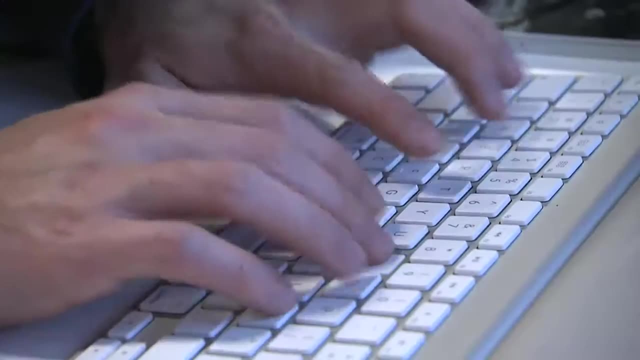 years of experience and are realizing. their undergraduate degree is fine, but it's a little bit too focused and they need to broaden. Since the program's first graduation ceremony, grads have already found exciting work in the thriving tech culture surrounding the University of Washington and beyond.